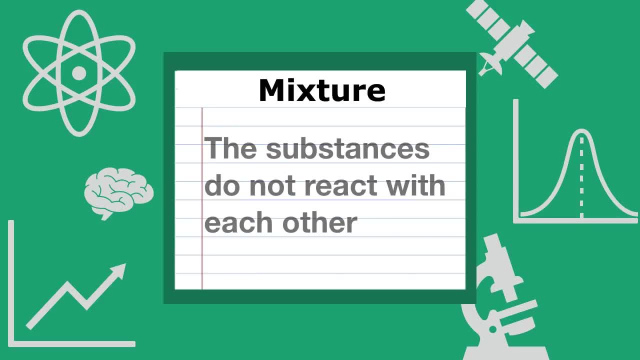 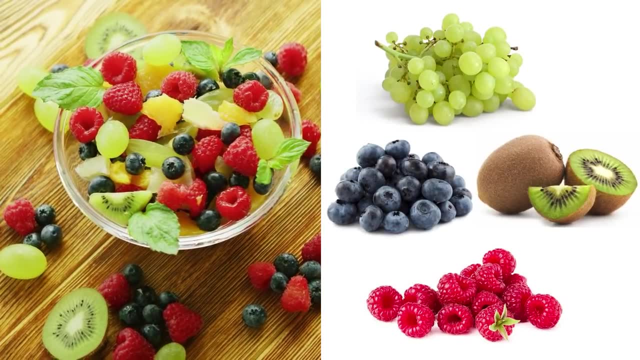 other fruits you'd like Now. a key feature of a mixture is that the substances do not react with each other. For example, in your fruit salad, nothing has changed about the fruit just because you've mixed it together. If you wanted to, you could separate out each individual fruit and see. 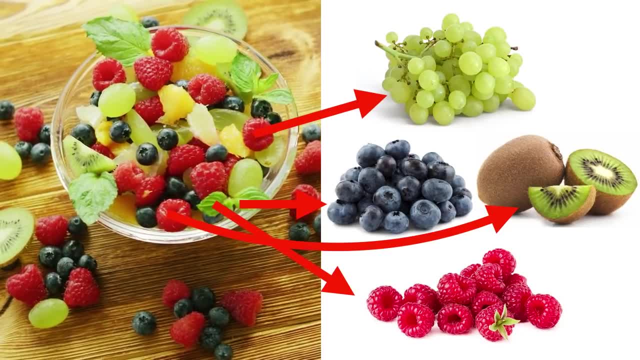 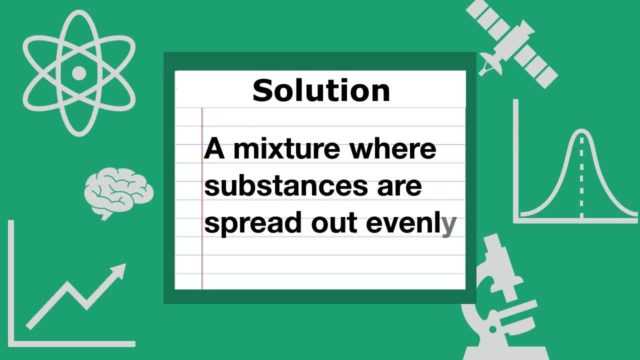 that nothing about it has changed. Now there's one more type of mixture. It's called a solution. A solution is a mixture where substances are spread out evenly. The best example of this is to think about putting a spoonful of salt into water. If you put the salt into the water and 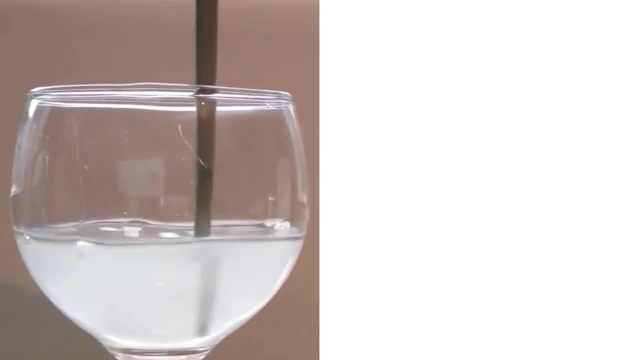 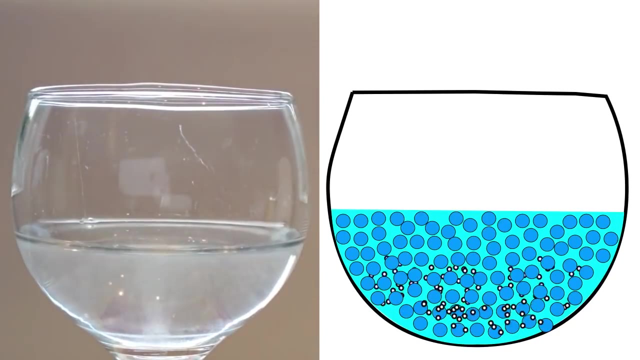 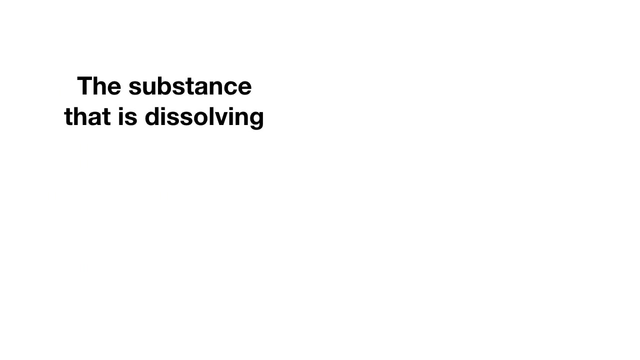 stir, the salt dissolves, making it look like it isn't there anymore. But what's actually happening when you dissolve salted water is that the particles of salt are spreading out evenly among the water. You just can't see them anymore. In solutions, the substance that's dissolving, which here was the salt, is called the. 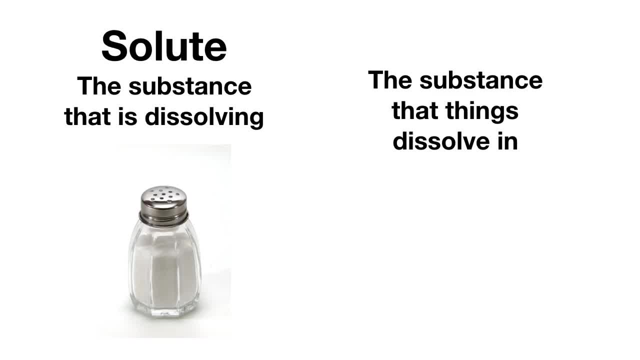 solute And the substance that things are dissolving, in which, in our example, was the water, is called the solvent. An easy way to compare mixtures and solutions is to think about taking a spoonful of each. If you were to take a spoonful of fruit salad one time, you might get a spoonful of blueberries. 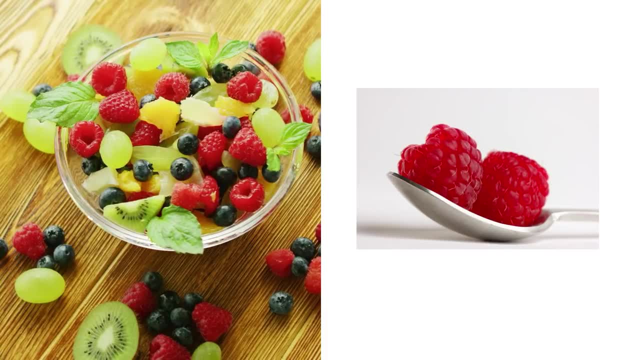 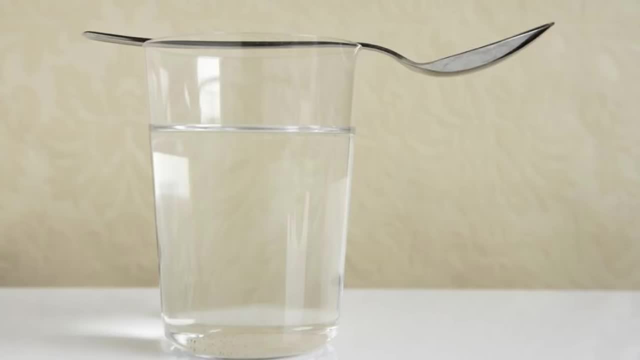 and the next time you might get a spoonful of contributing salt. Then you could have different of raspberries. Each time you take a spoonful it would be a little bit different, But in a solution like salt water every spoonful you would take would be just as salty. There will be no extra. 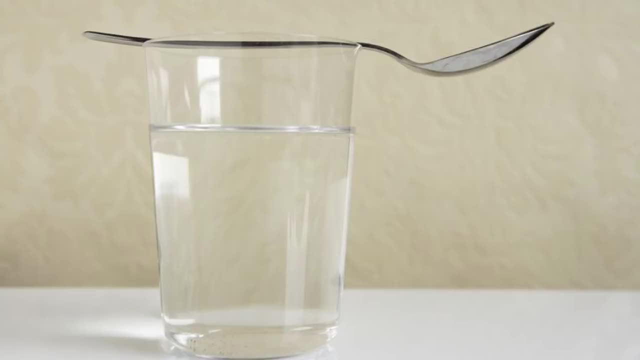 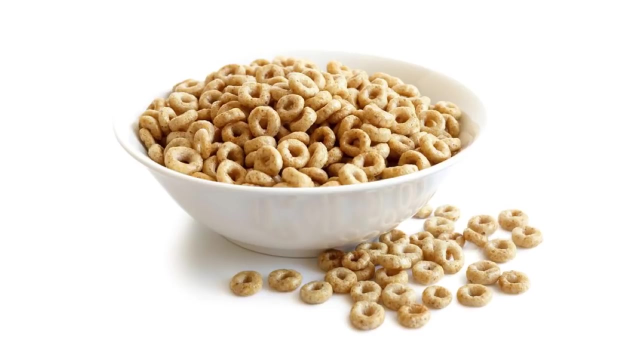 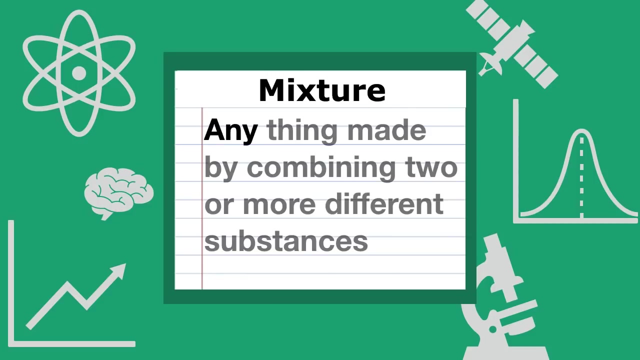 salty spoonfuls, because it's all mixed evenly together. Now let's practice identifying mixtures and solutions together. Let's start by deciding if this bowl of Cheerios represents a mixture solution or neither. Well, what is the definition of a mixture? Remember that a mixture is anything. 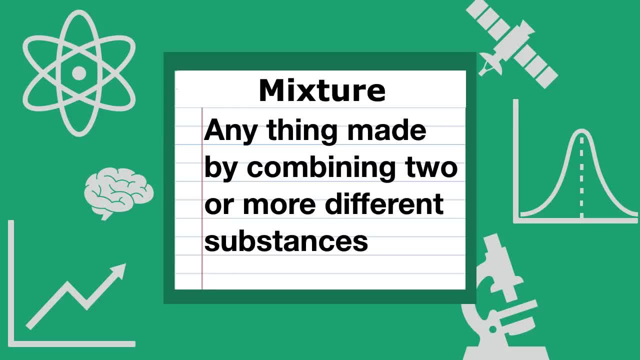 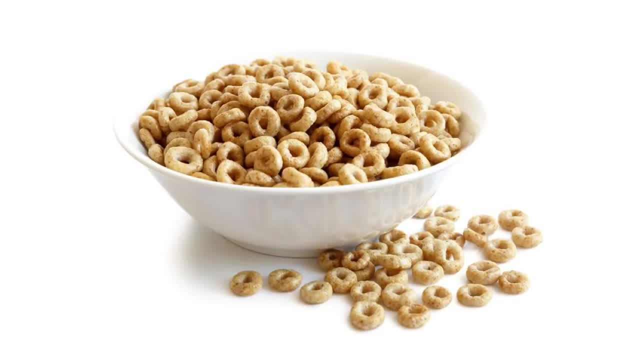 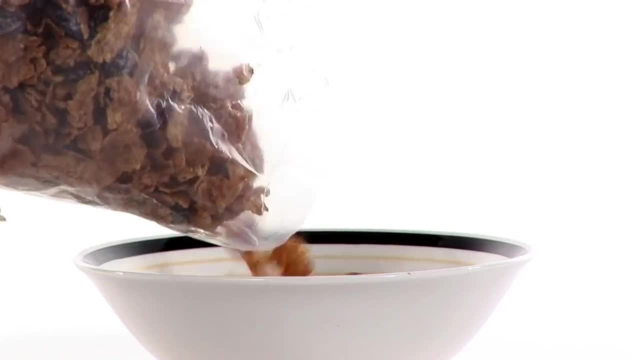 made by combining two or more different substances. And in our bowl of Cheerios- assuming there is no milk- do we have two different substances? No, all that's in this bowl are Cheerios, so this is neither a mixture nor a solution. Now let's look at another bowl of cereal. 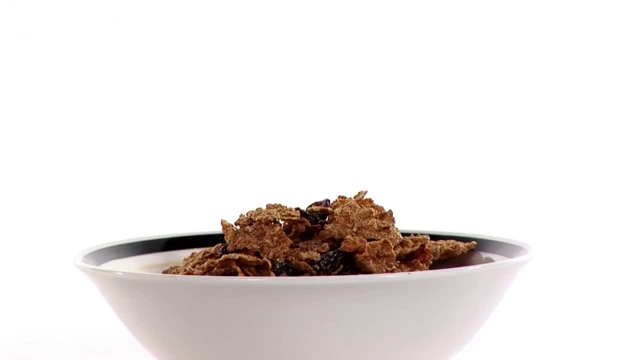 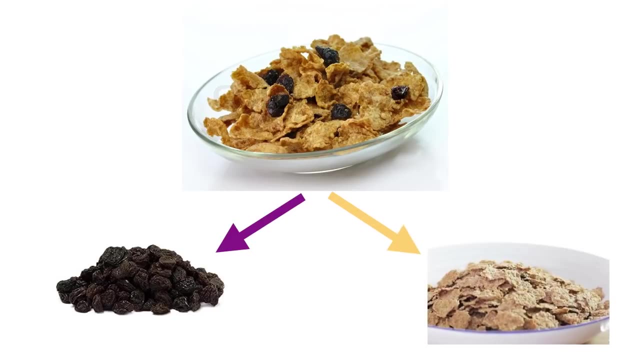 Imagine pouring yourself a bowl of Raisin Bran. Well, what is being mixed together in a bowl of Raisin Bran? Well, Raisin Bran is made by mixing together both raisins and cereal. So what is Raisin Bran?